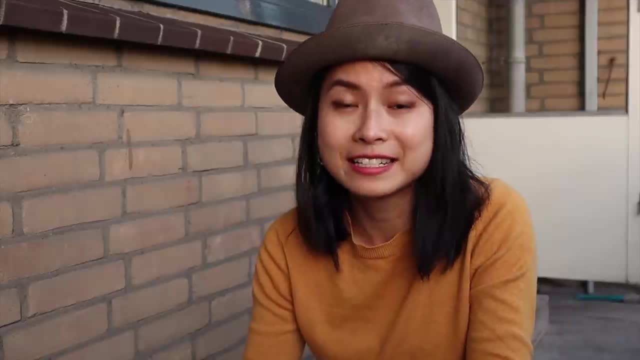 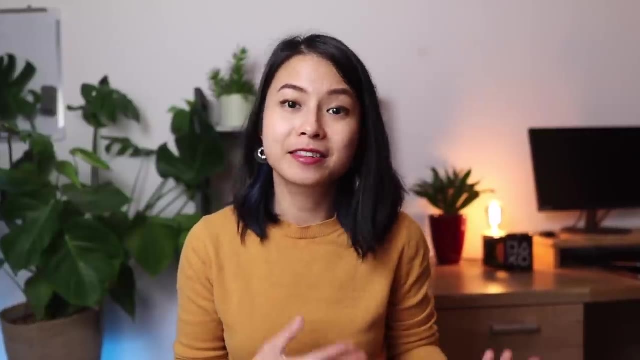 a house using these tools. This includes the core knowledge, such as business knowledge, math, statistics and statistics. This includes the core knowledge, such as business knowledge, math, statistics and statistics, modeling and design. most of us might find ourselves being better at the tools. 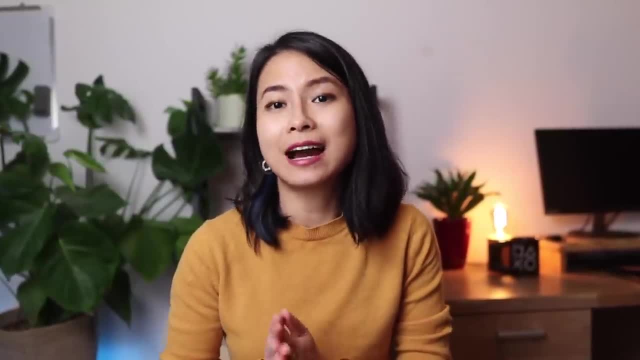 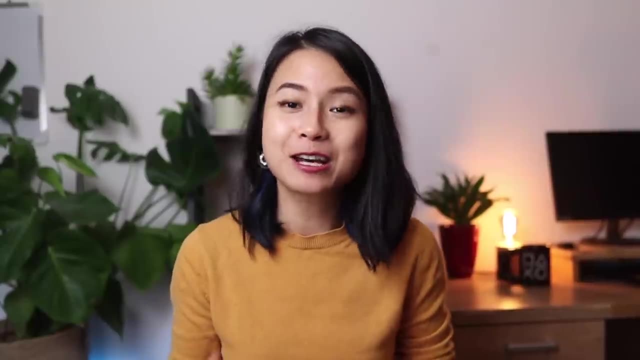 than at the other things, or vice versa. I think a good book would ideally cover both theories and tools, but more often than not they are dedicated to only one or the other, and this is totally fine. you just need to be aware of that and know how to complement learning from different books. so, for each book. 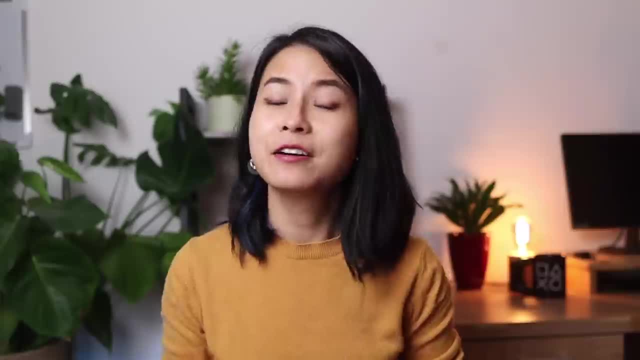 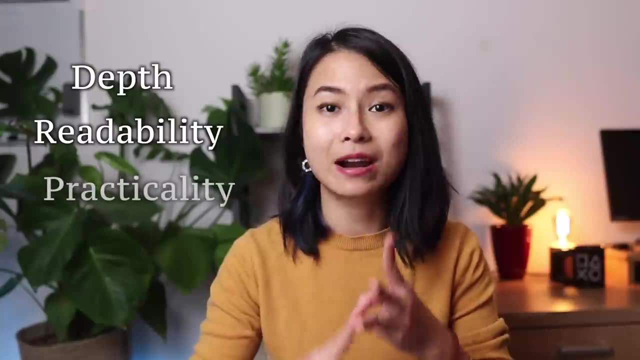 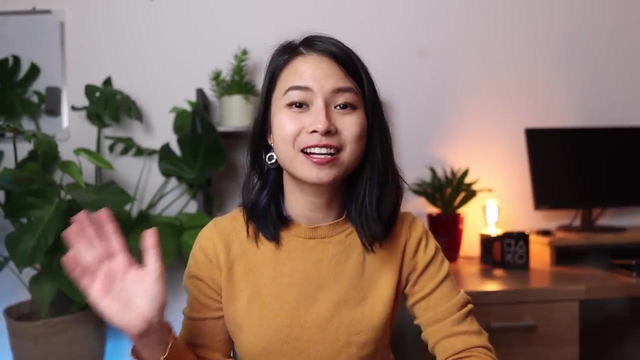 mentioned this video. I'll rate them using three criteria. firstly, depth: does the book cover the topic in depth? second, readability: is it easy to read? and finally, practicality: can the knowledge from the book be easily applied in practice? without further ado, let's dive right in the first book I start with is 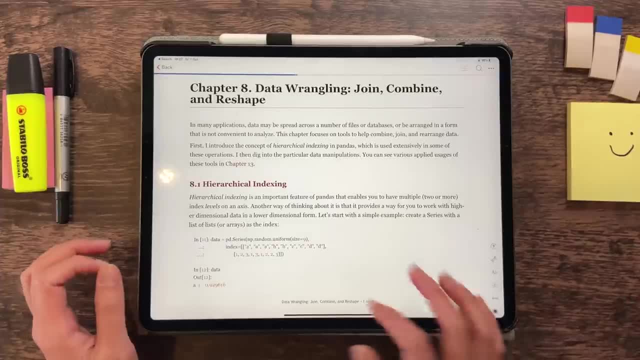 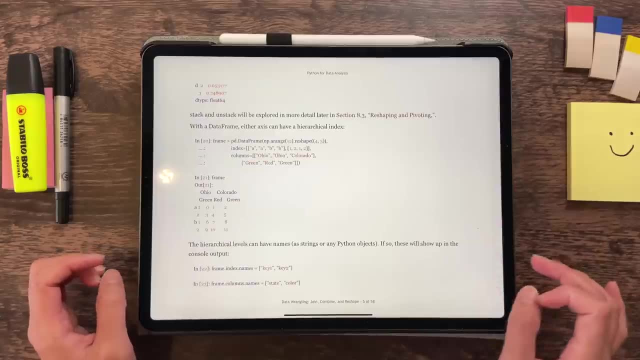 Python for data analysis. this book is mostly about pandas, numpy, matplotlib and, additionally, scikit-learn and stats model. I have it on my iPad because I want to be able to copy paste the code and check out the web links from here. you might have been familiar with these. 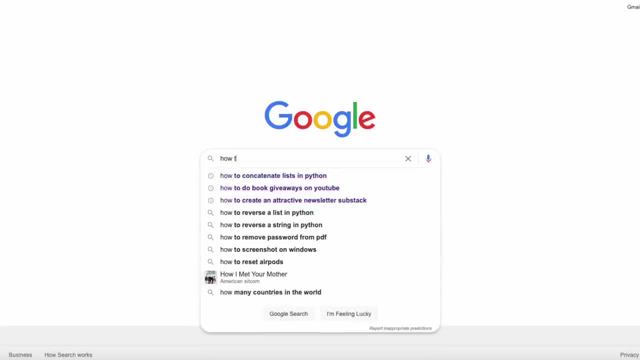 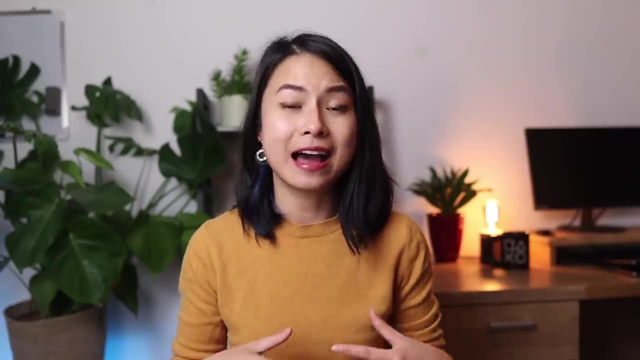 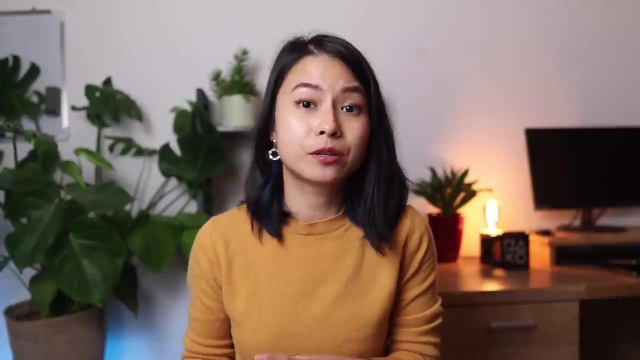 libraries. in my case, I learned a ton just from googling and using snippets coupled together from dozens of stackoverflow threads. however, with this book, it's nice to have the material in a clear, thoughtful and organized way, so it can be a very good reference that you can use in conjunction with an actual 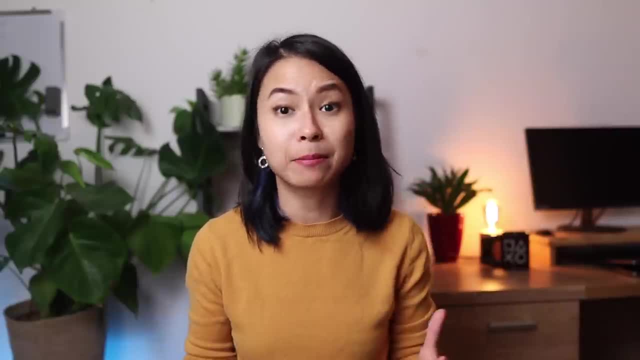 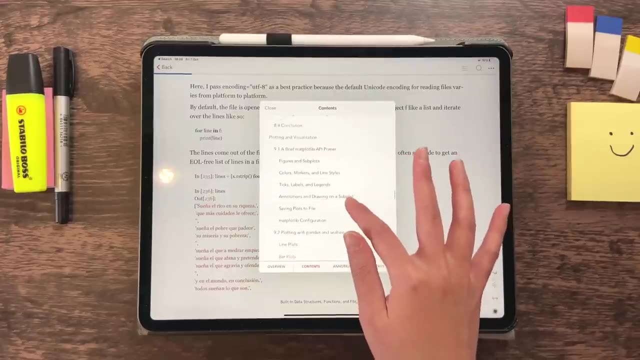 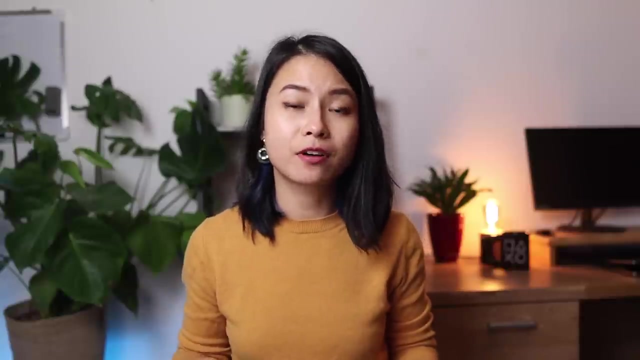 Python course you're taking and help you fill in some gaps you may find in the courses. there are 13 chapters in this book covering from basic Python setup, basic data structures and syntax, and data cleaning and transformation with pandas and numpy. it also has dedicated chapters for plotting and visualization, time series and 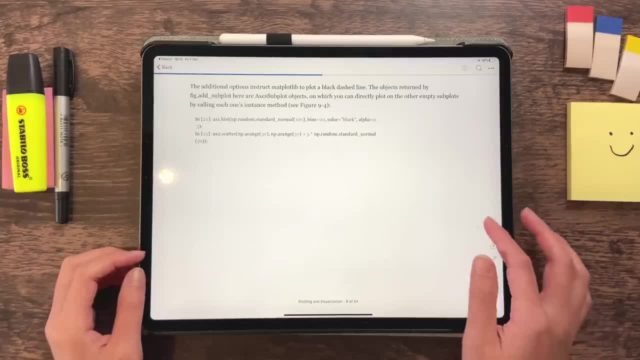 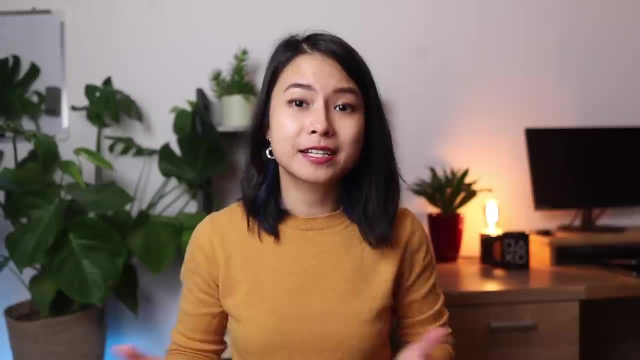 modeling. this book has a lot of code examples for a lot of different types of data wrangling and analysis and explains many common gorgeous for new python users. the book doesn't cover more advanced topics such as polarization, object-oriented programming, so overall I'd give this book 4 stars for Concept시. 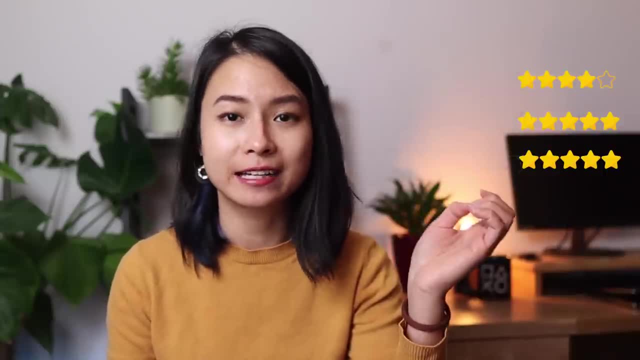 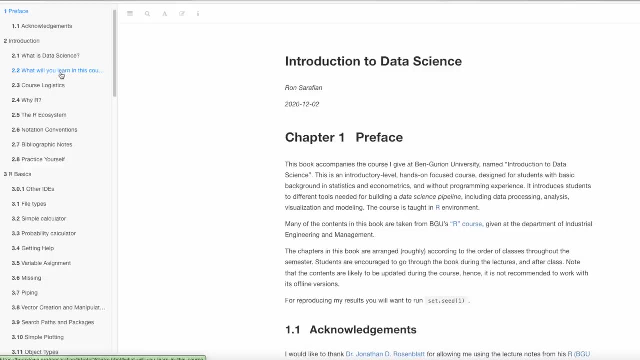 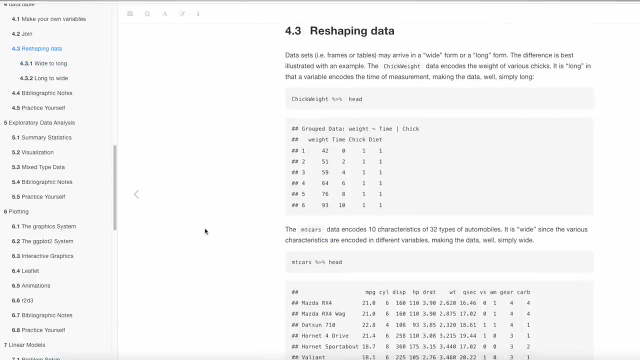 5 stars for Readability and 6 stars for Mathematics. stars for practicality. if you're learning r for data science. instead, an equivalent introductory level book i found is an online book called introduction to data science by ron seraphian link in the description. it's beginner friendly but dangerous enough to teach you really useful stuff. 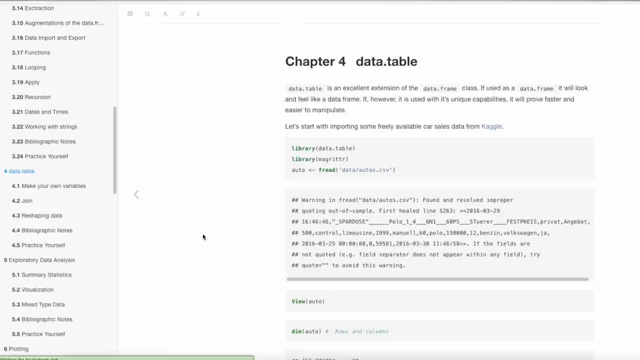 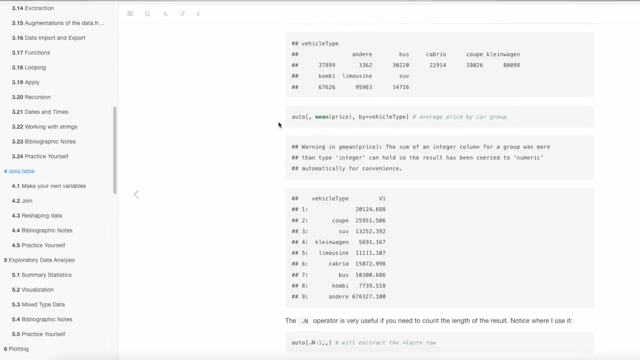 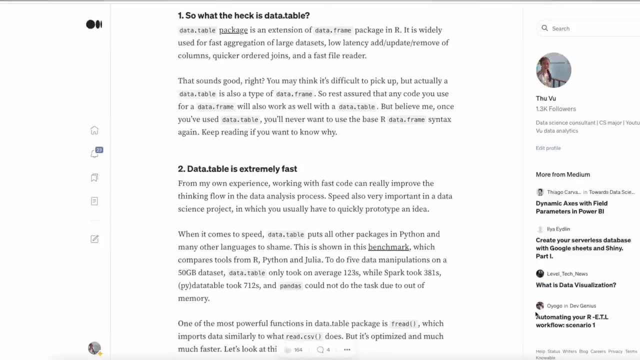 actually it's the only r book i found that uses datatable, which is a library in r. that improves the performance and simplifies a lot of the clunky base r data frame syntax and honestly, i love r datatable even more than pandas. i wrote a whole article a while back about it, but please don't. 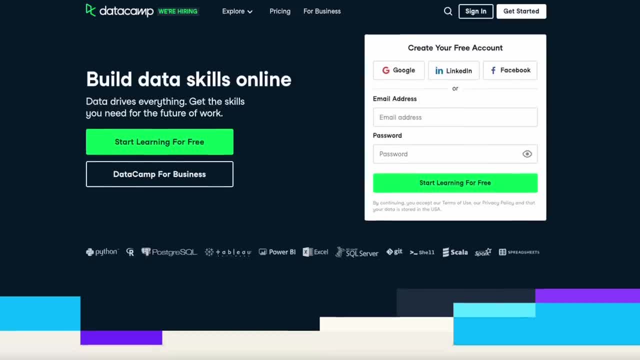 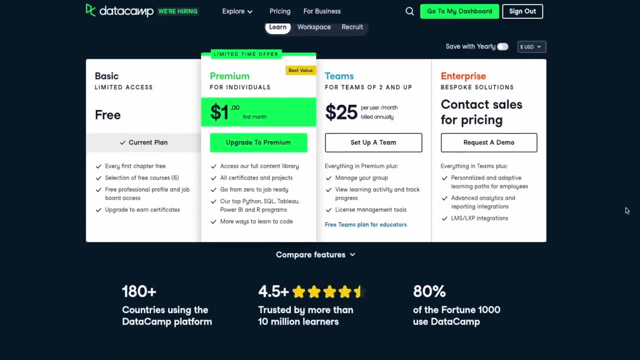 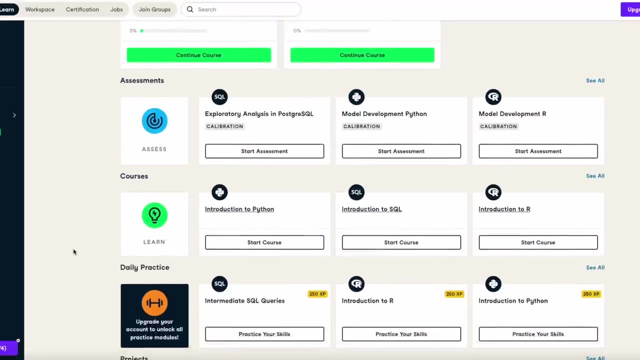 hate me for this, talking about learning python and r. datacamp is running a week-long promotion to commemorate world space week. so between october 3rd and october 9th, learners can pay just one dollar for a month's worth of unlimited content of datacamp's entire learning platform you can take. 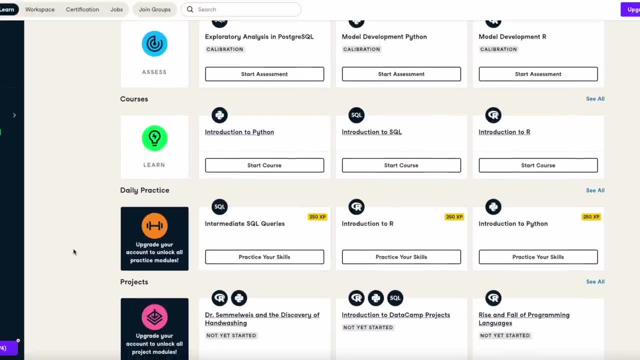 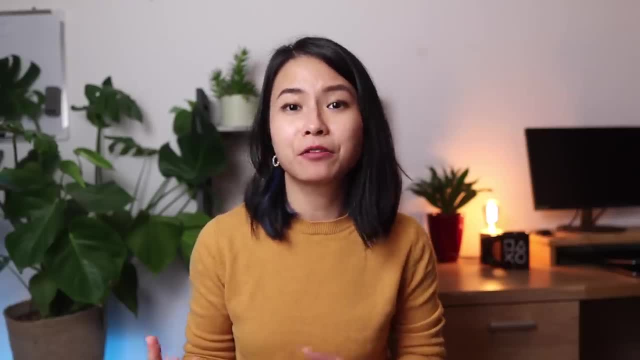 any courses you like on the platform, from python, r to data analysis with powbeye, after a month of training and you will have a public course for the whole day. it's free and you will also receive. if you enjoy the courses and would like to continue the subscription, you pay full price. 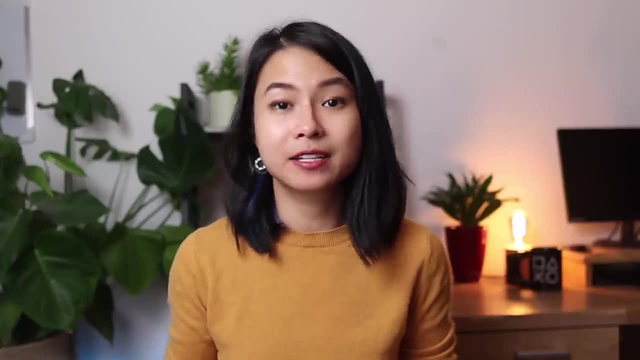 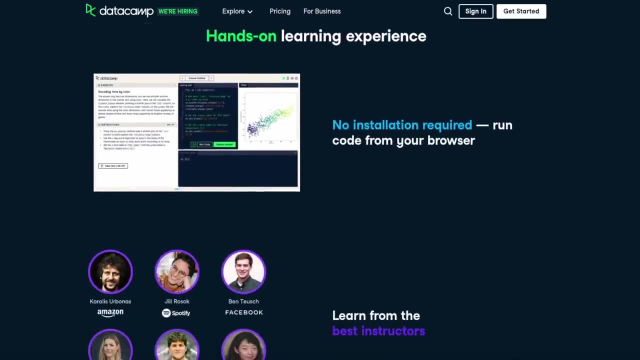 per month going forward. Compared to Coursera, Datacamp doesn't provide certificates, but it lends itself to the more practical approach to teaching. You can code directly on the platform and follow along with the lessons, which is perfect for beginners who don't want to have to install. 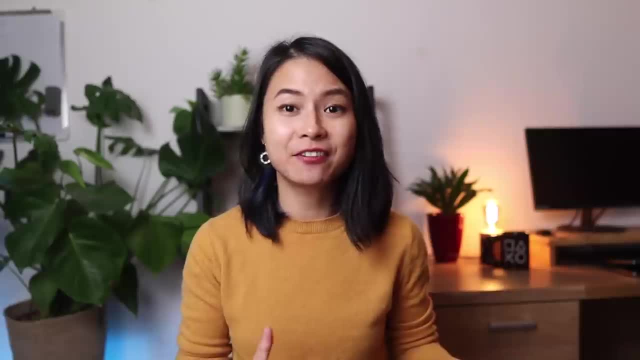 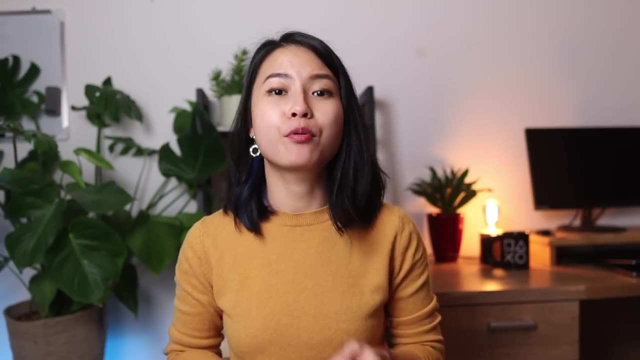 the software yourself. You're basically taken by the hand to learn stuff. If you're interested, check out the link below. Thanks to Datacamp for sponsoring this video. Moving on to statistics books, I think Practical Statistics for Data Scientists is the most useful and beginner-friendly. 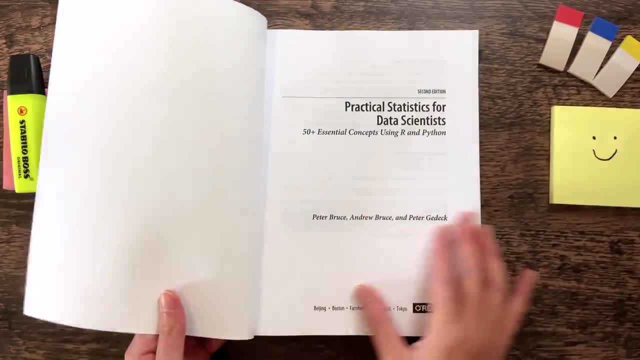 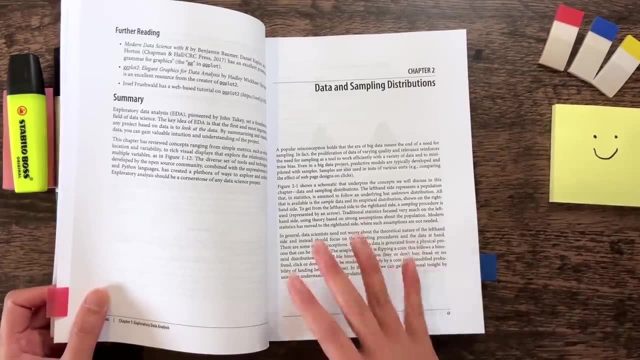 one. It covers all the core concepts that you need to know for data science, including descriptive statistics, sampling distributions, hypothesis testing and A-B testing, and prediction and unsupervised learning. Actually, for one of my earlier videos about statistics for data analysis. 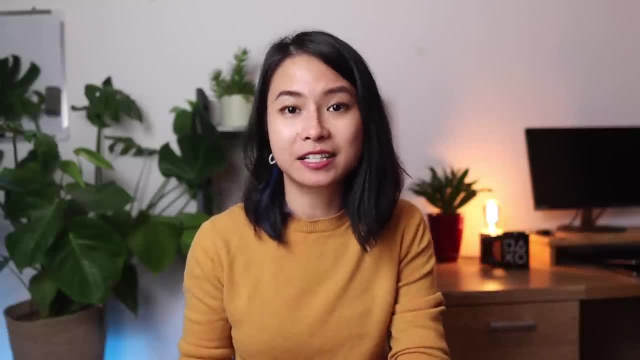 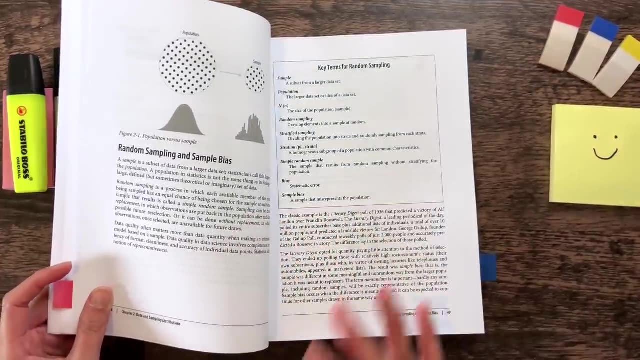 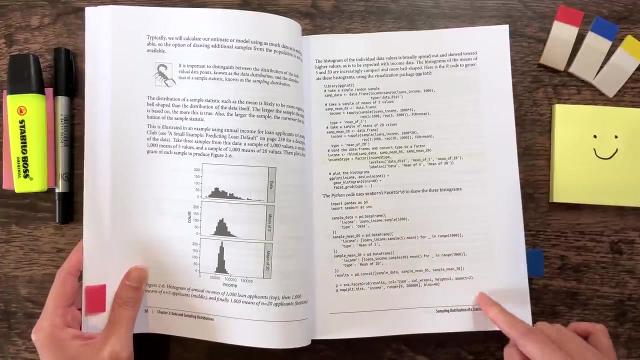 I draw a lot of inspiration, and the key content items form the first two chapters in this book. Each statistics concept is delivered very concisely in bite-sized sections with the key ideas and key terms you need to know, in a very approachable way. Each concept also comes with a code snippet for both R and Python, so it's quite. 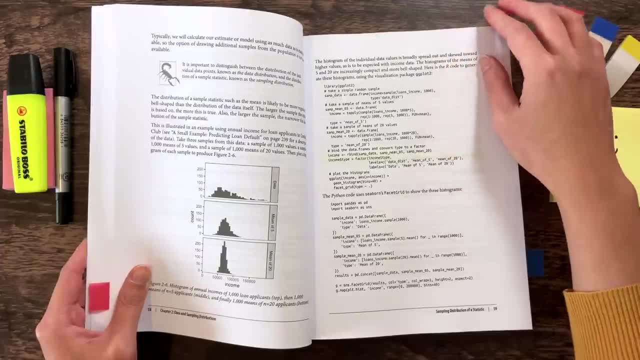 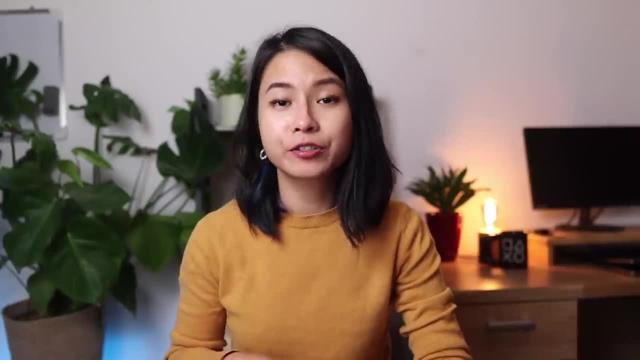 handy to test out the code yourself and see how things work. This will help you to quickly connect the theoretical concepts with the practical use. If you want to read further on a topic, there's a section for further reading. It's really one of the most practical and approachable books about statistics for data. 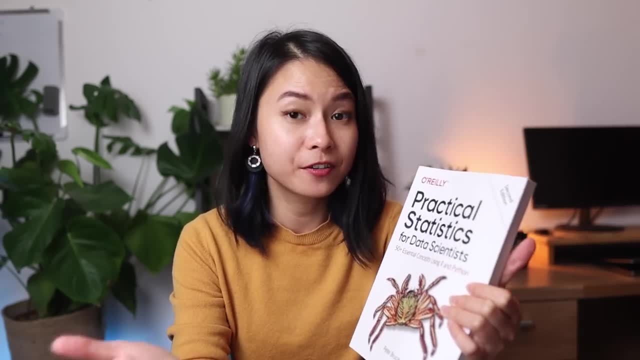 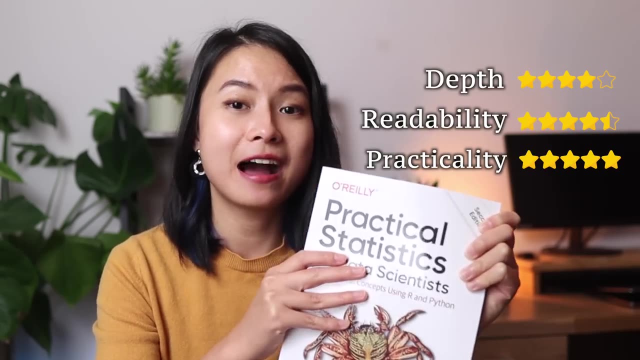 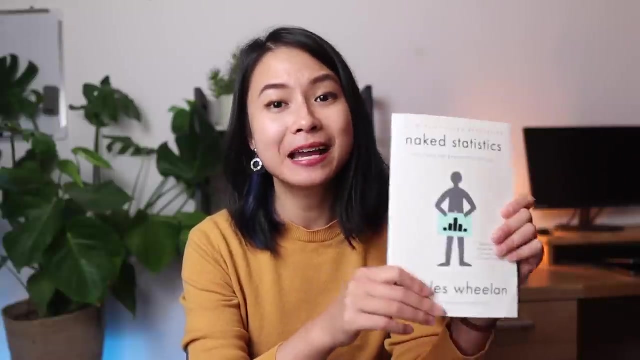 science, I've found, although some topics could be discussed further in depth. so I'd rate this book with 4 stars for depth, 4.5 for readability and 5 for practicality. A super casual and fun book, for Statistics 101 is Naked Statistics. It explains the fundamentals. 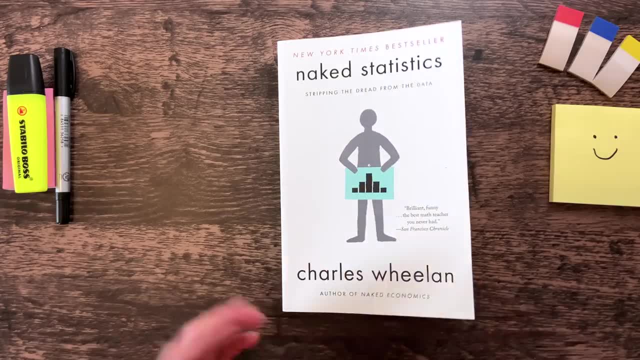 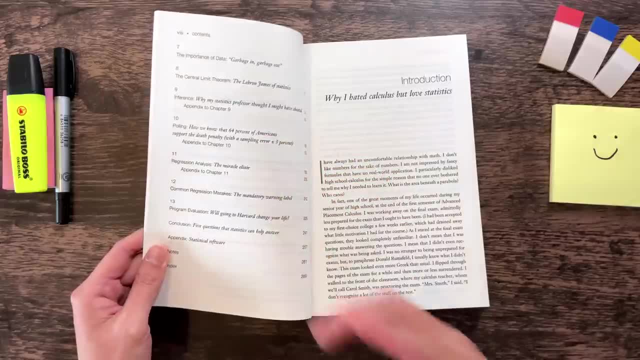 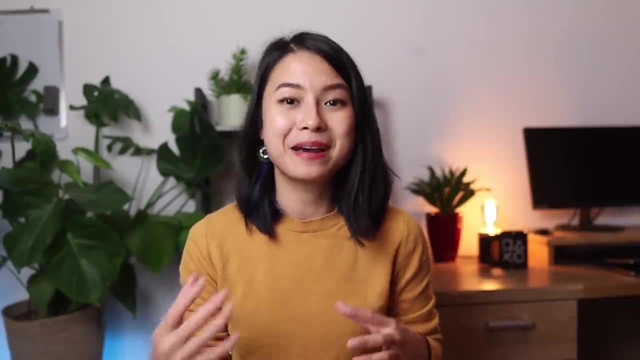 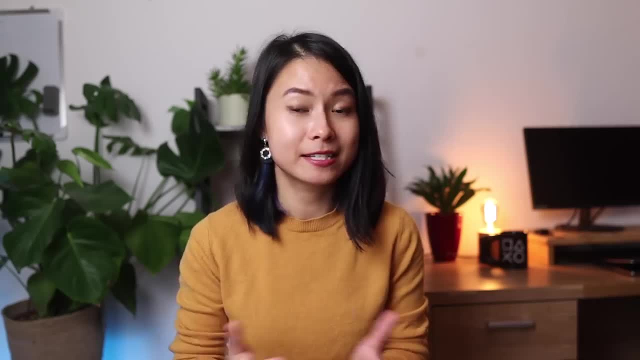 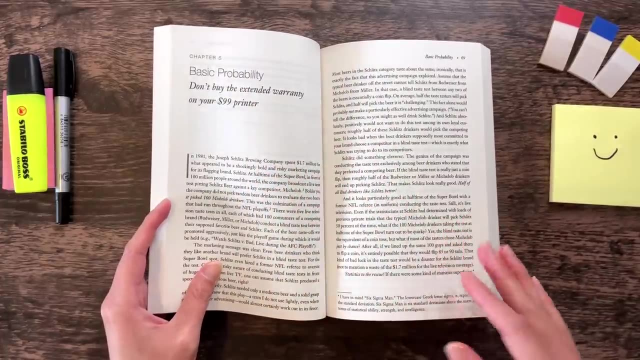 mistakes we make, from big to small, when it comes to statistics and modeling. One of my favorite chapters is: Don't Buy the Extended Guarantee on Your $99. Printer. I must have laughed in tears reading this chapter because it reminds me on the first lesson I got about personal finance. 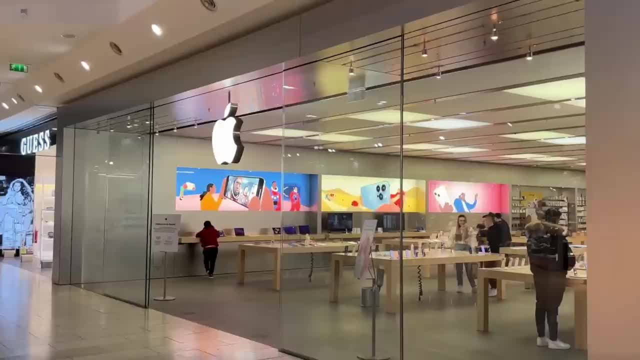 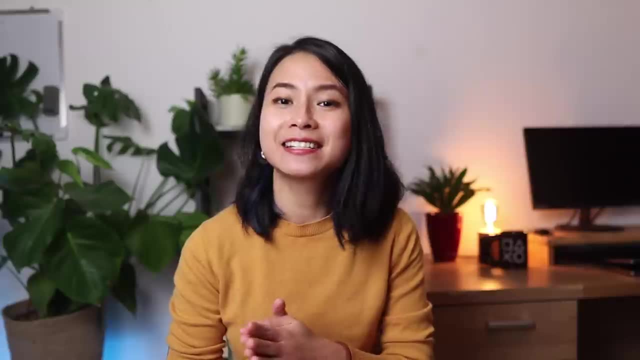 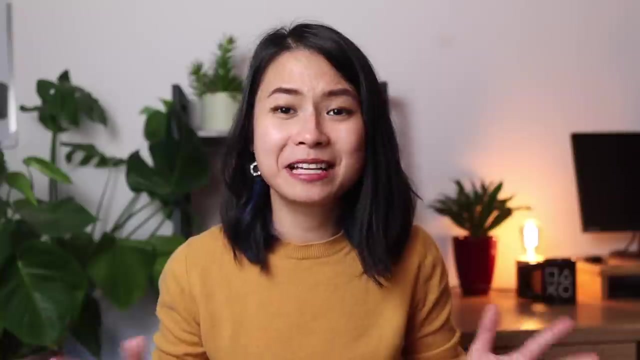 when I got my first job and maybe the first paycheck, I went on to get myself a new iPhone at the store for like $500.. At the checkout, the sales assistant asked me if I want to buy a phone insurance in case of theft or if the phone breaks down Somehow. I thought it made a lot of. sense buying insurance for my beautiful new phone. Then I went on to buy the one-year insurance plan that cost $7 a month. I came home that day, after all the shopping frenzy, I sat down and realized: oh no, it was such a terribly stupid idea. Who on earth would pay $80 of insurance a year for? 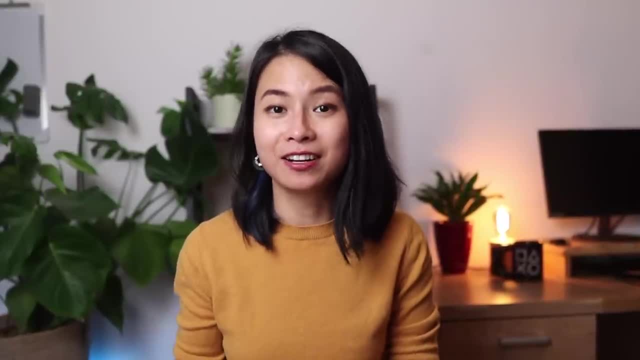 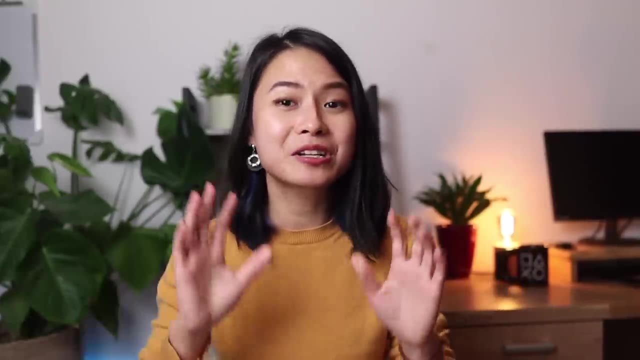 a $500 phone when the chance of having my phone stolen is one in thousands. No wonder the sales guy was so sweet to me. So lessons learned from the chapter is that you should only buy insurance for things you can't afford to withstand, if something bad happens, like your health. But 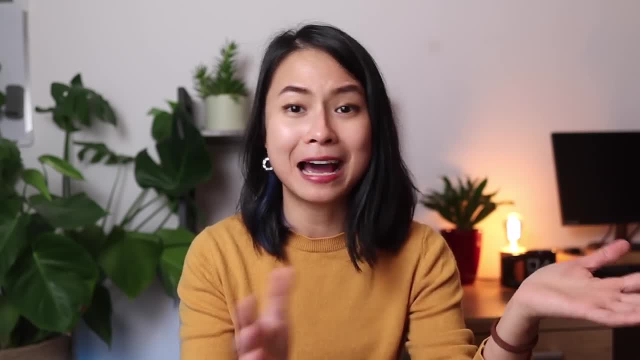 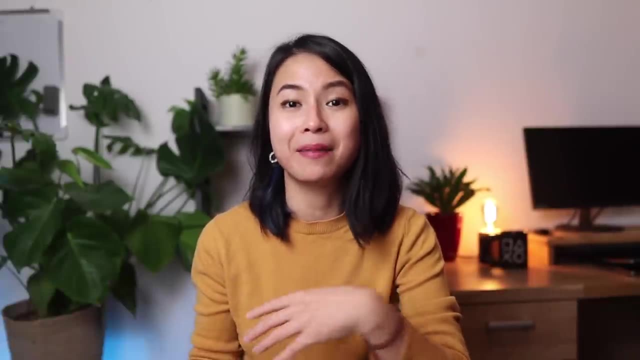 other things, like your $99 printer and other appliances. they are the last things you want to buy insurance for. This is how insurance industry uses probability to make money. A pity, I must say, is that this book doesn't cover Bayesian statistics, but it's overall a very good. 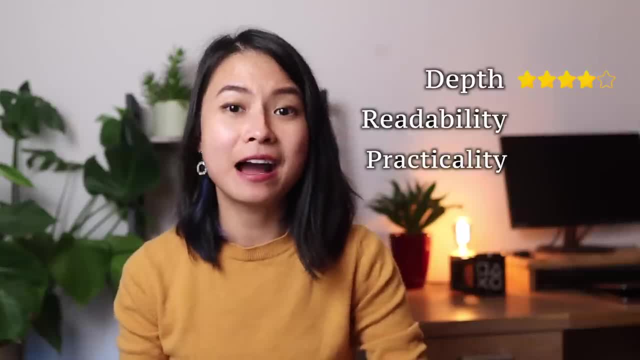 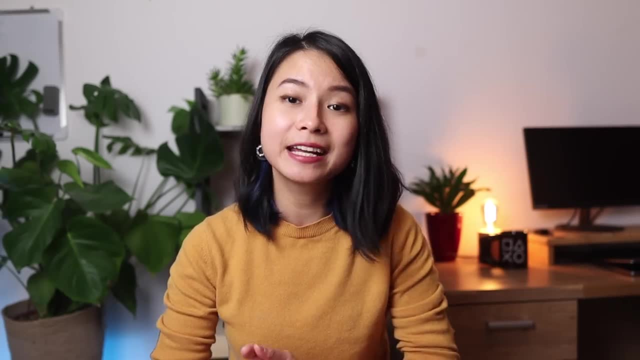 entertaining book, So I'd rate it 4 stars for depth, 5 for readability and 5 for practicality. Regarding math books, math I think is mostly required for machine learning, For common data analysis. you generally need a good math book, So I'd rate it 4 stars for depth, 5 for readability. 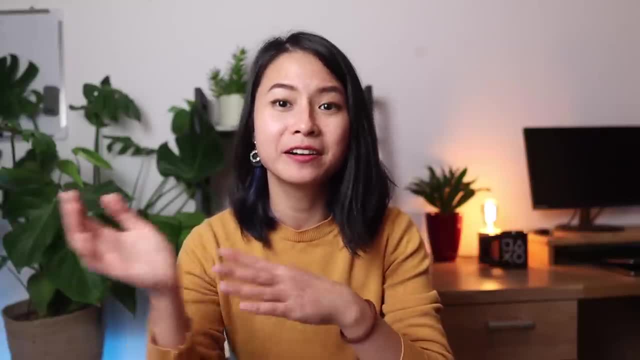 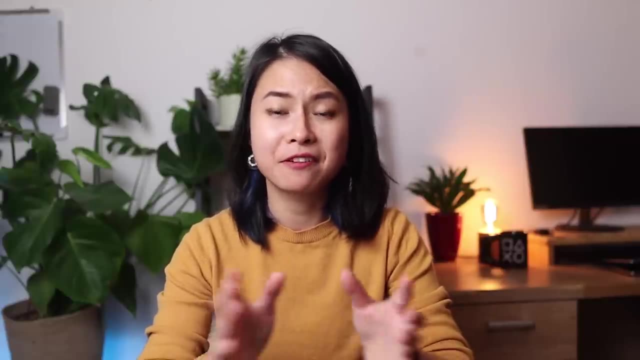 very limited amount of calculus or linear algebra For learning essential math concepts. I wouldn't recommend reading books as starters. Most math for data science books I found are pretty hard to read for beginners and even straight out boring. So I'd actually recommend 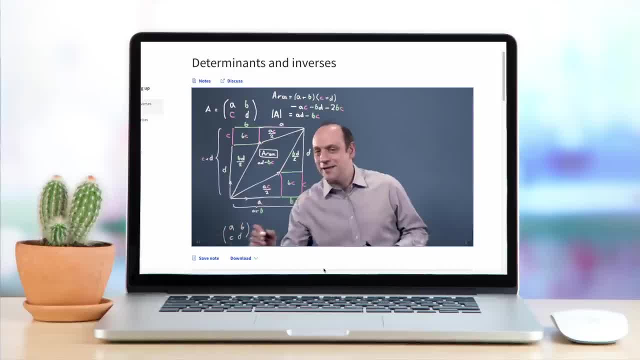 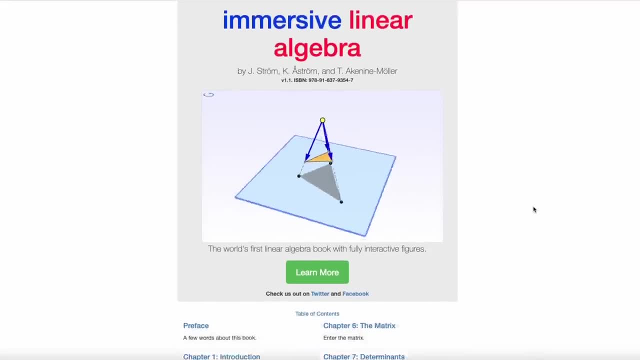 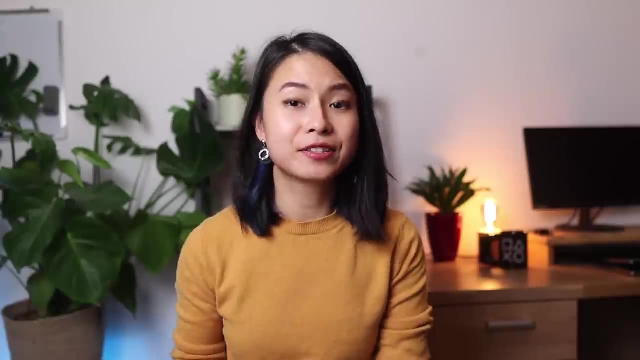 you first taking an online course to have the basic of calculus and linear algebra under your belt. In combination with that, you could use the interactive books, such as immersive math, and explain it visually. I've linked to the website in the video description below. I actually only use math books mostly to 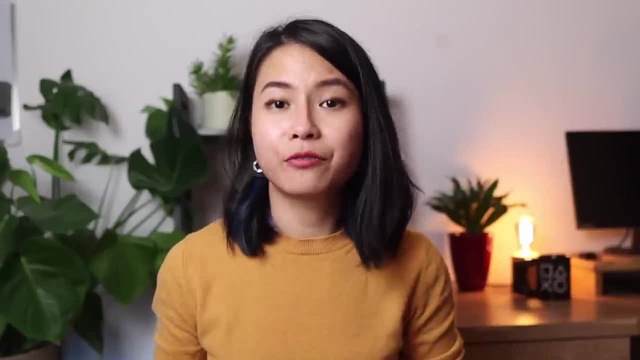 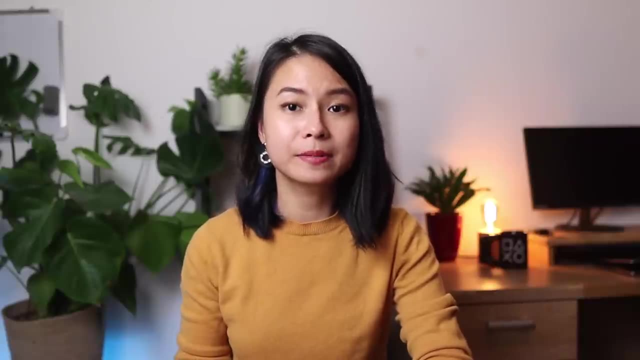 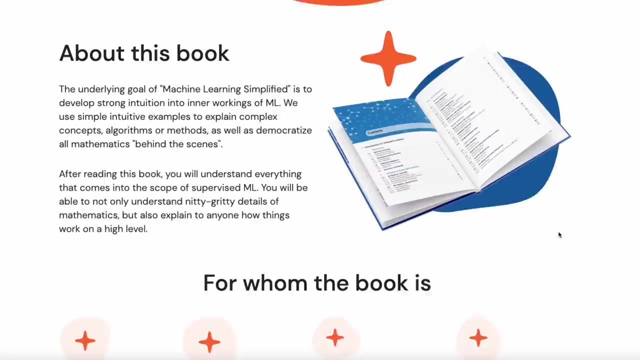 look up for the formal definition of something. When you feel ready and comfortable with fundamentals, there are some machine learning books that helps you learn pretty well the math behind the algorithms. For a truly gentle introduction to machine learning, I'd recommend Machine Learning Simplified. It's a new book that was published earlier this year that covers the 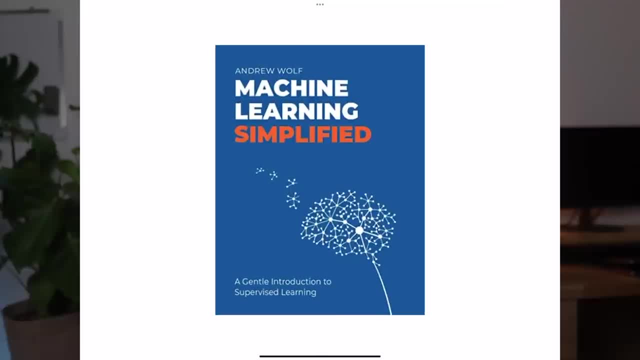 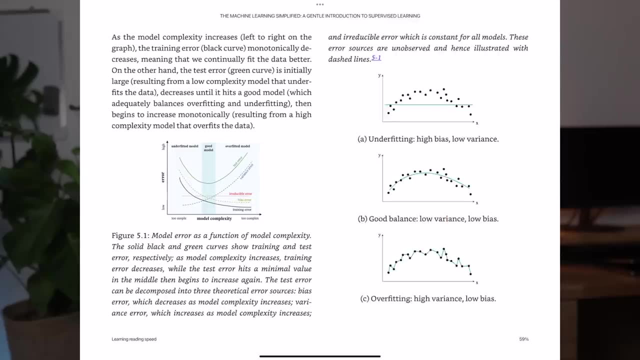 fundamentals of machine learning. It's a beautiful book and I must say I'm pretty impressed. I'm impressed at how much ground this book covers and how accessible the topics are presented. You can read the first few chapters for free on its website or get the ebook for just $2 on Amazon. 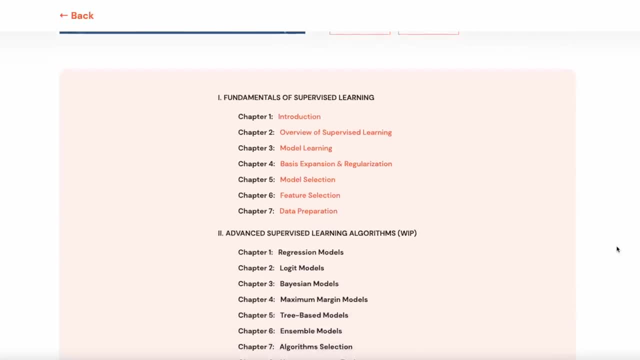 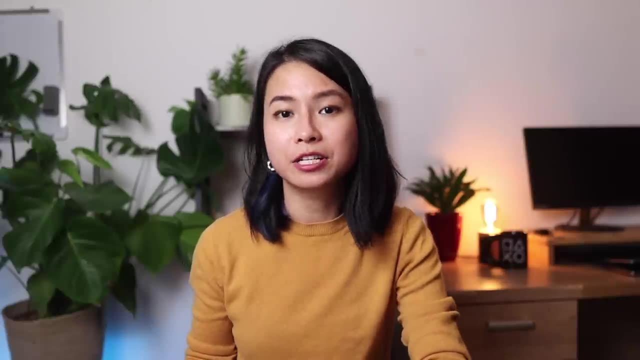 which is totally insane. The second part on unsupervised learning is still coming, I think. So I think this is an excellent book, whether you're new to data science or need a refresher, because it's very easy to understand and realize more on intuitive examples to explain the concepts. instead of only showing you the basics. I think it's a great book to read if you're new to data science or need a refresher, because it's very easy to understand and realize more on intuitive examples to explain the concepts instead of only showing you the basics. 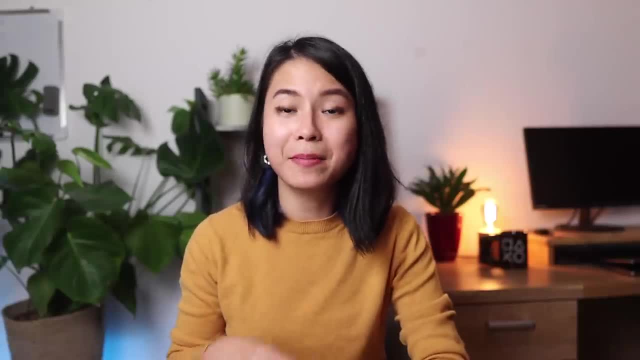 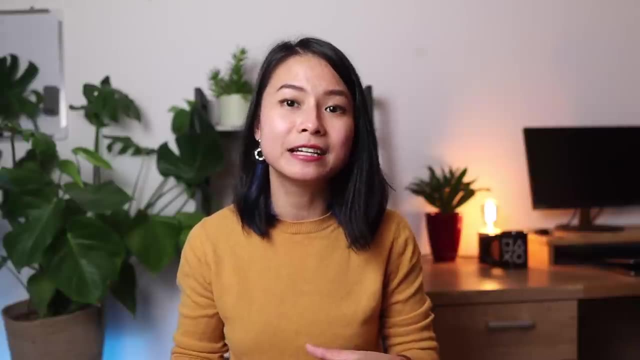 So far. I think this is one of the best introductory machine learning books I've found. that gives you the exact portion of knowledge you need to know as a beginner, so you don't feel overwhelmed. The book also has a repository that contains the actual Python implementations. 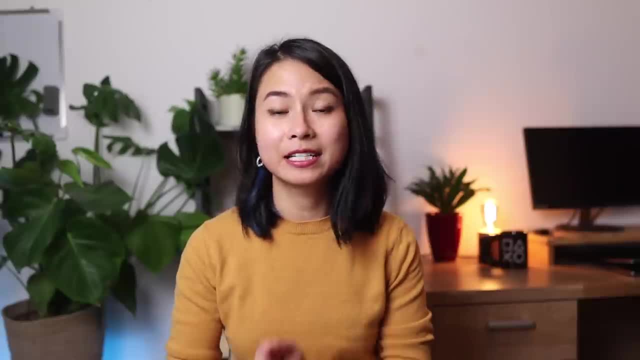 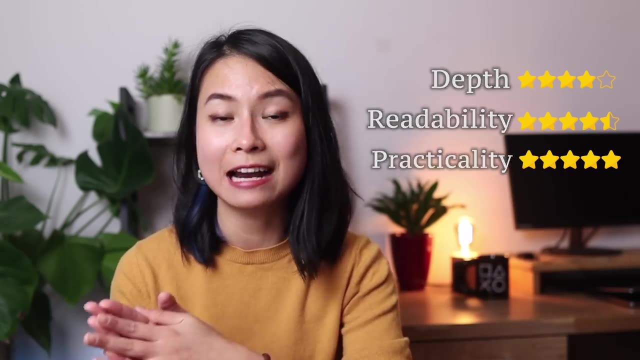 of all the topics discussed in the book. It's a great book, very inexpensive. I love it. I'd give this book 4 stars for depth, 4.5 for readability and 5 for practicality. The next book on machine. 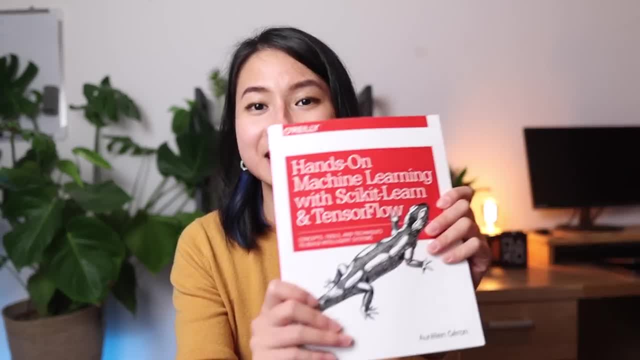 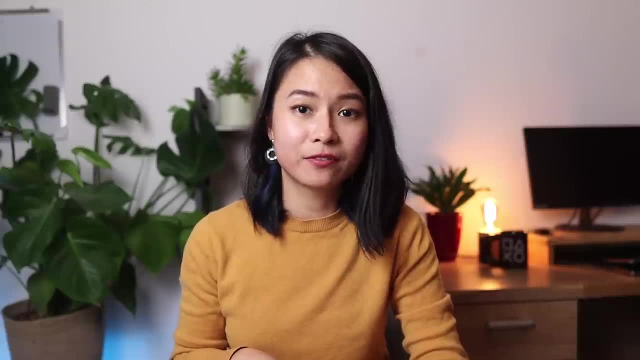 learning that's loved by many people is Machine Learning with Scikit-Learn and TensorFlow. I've got the first edition, and the second edition looks a bit like this: This is, I think, the best book of its kind for data scientists and machine learning practitioners. The book has two parts: the 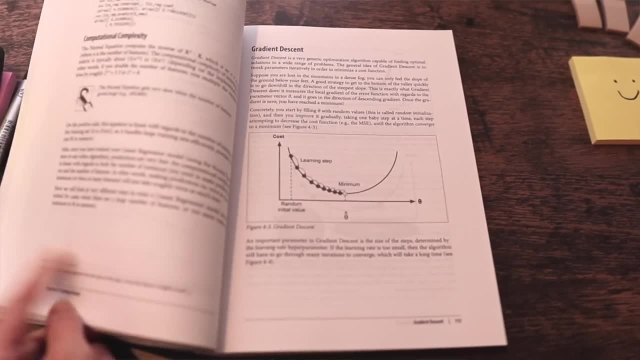 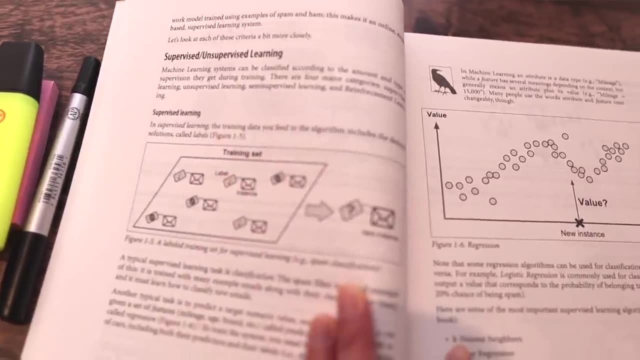 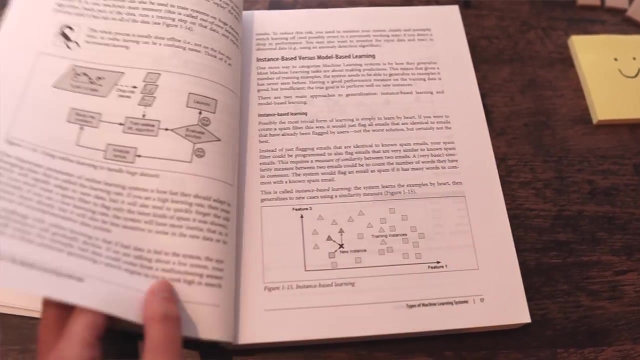 fundamentals of machine learning, and part two is about neural networks and deep learning. The book first starts with an overview of different machine learning systems, the common challenges in machine learning, and then it goes on to data transformation and how to train models, and all the different techniques, terminologies and metrics you need. 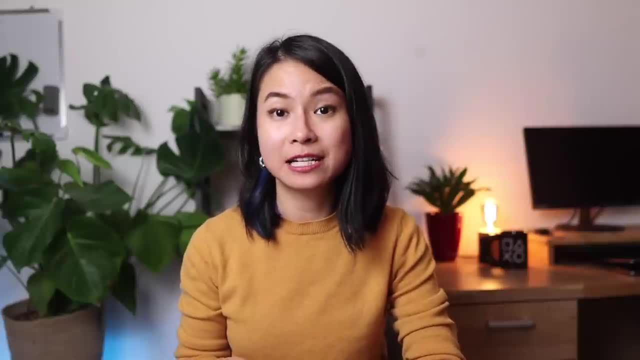 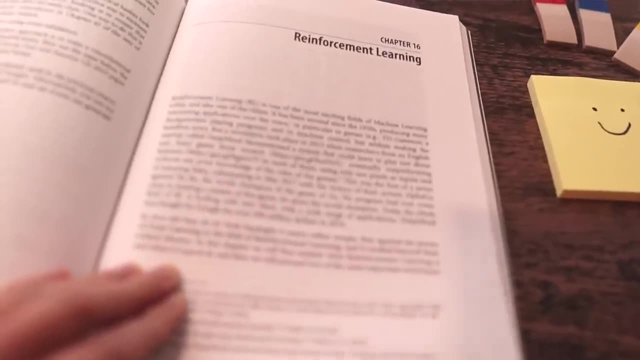 to know. You can find all the most common supervised machine learning algorithms here. Part two covers building deep learning models with TensorFlow, and at the end we also have a small chapter on reinforcement learning using OpenAI Gym. Exactly as the name suggests, this is a very 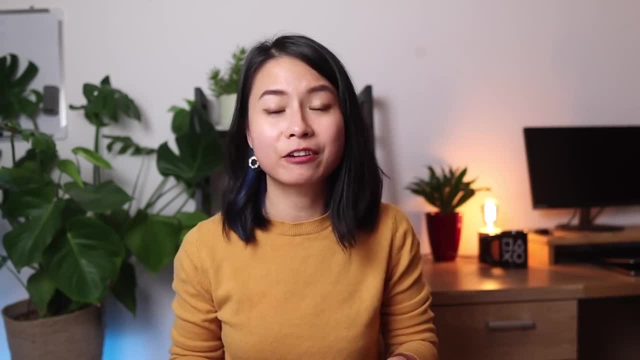 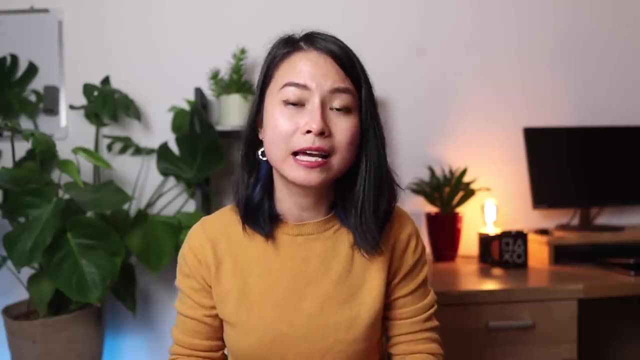 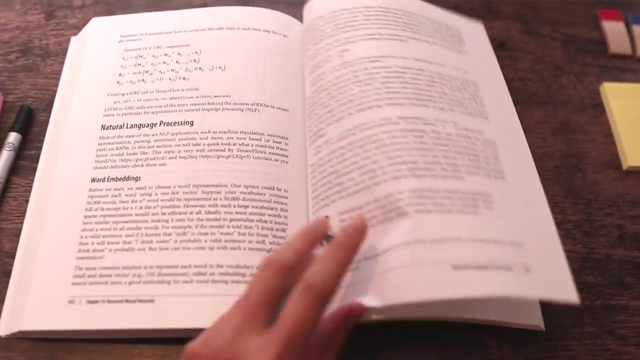 hands-on book. for each machine learning concept or algorithm that the book introduces, There's a page explanation of what the concept is about in a nutshell. Then the book dives straight into the implementation of the algorithm with Scikit-Learn in Python. I really love the tone and the language. 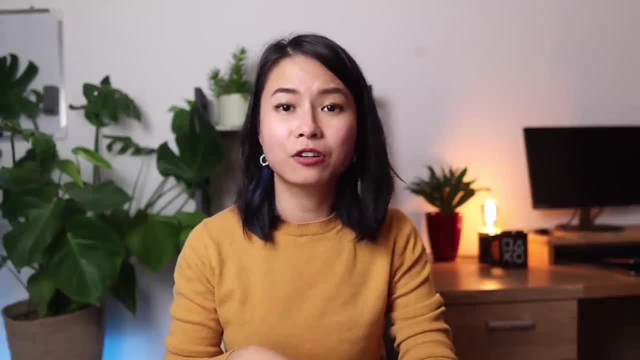 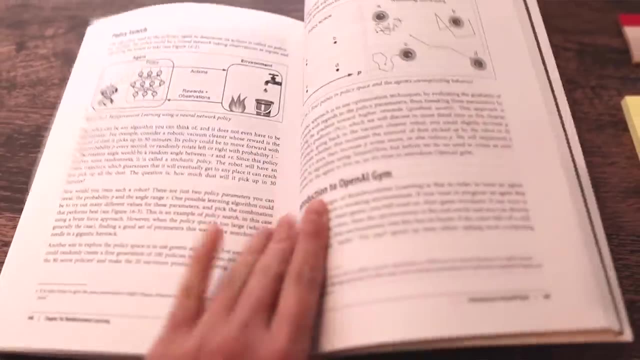 used in the book. There's really no jargons and even difficult math formulas are used very sparingly. The book lends itself to a more intuitive approach with simple English. Also the data, example pictures and diagrams to help you gain a high overall understanding of the. 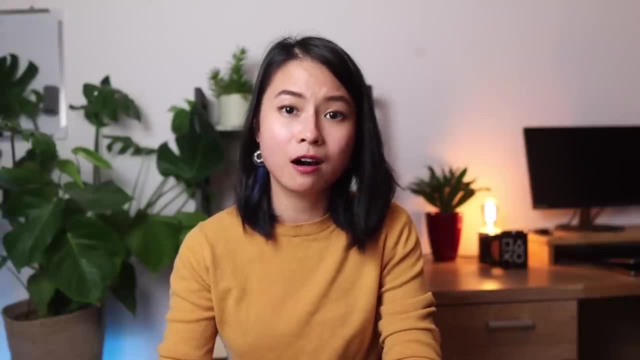 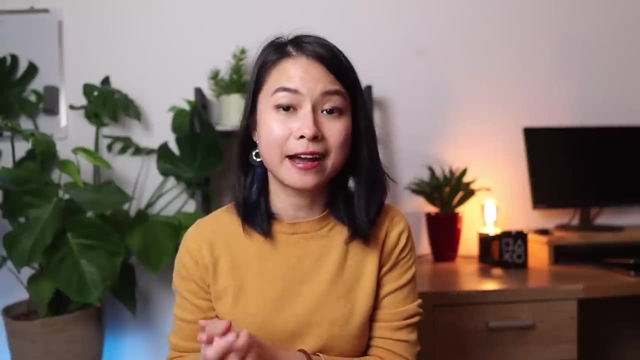 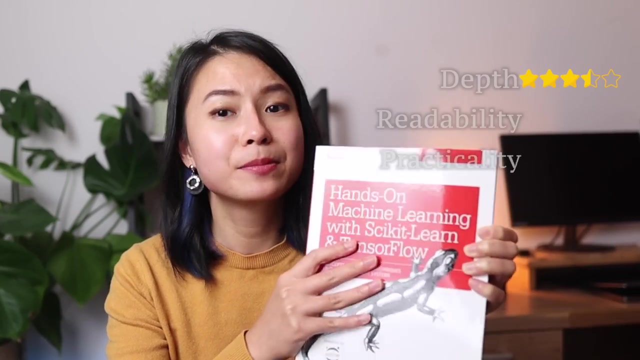 concept. However, I feel like there should be more discussion on comparing and contrasting different algorithms and example cases in which an algorithm might be more preferred than others, or which algorithms are being used in practice by companies in industries. So I think I'll give this. 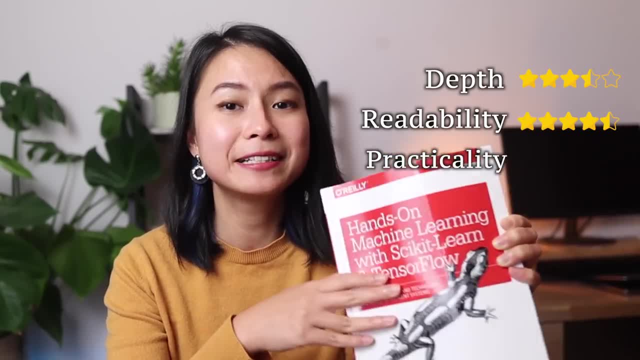 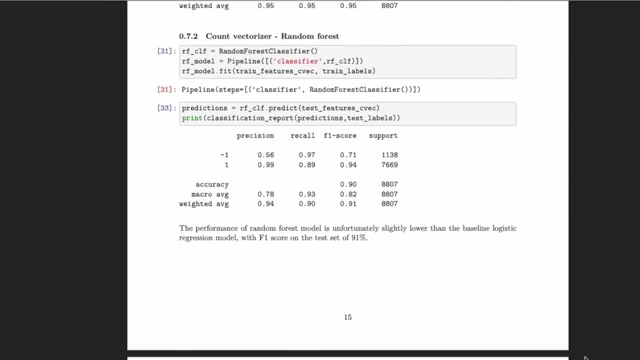 book: 3.5 stars for depth, 4.5 for readability and 5 for practicality. There's often a big gap between developing machine learning models in Jupyter notebooks with actually deploying and scaling that model, So I think it's a good idea to give this book a try. 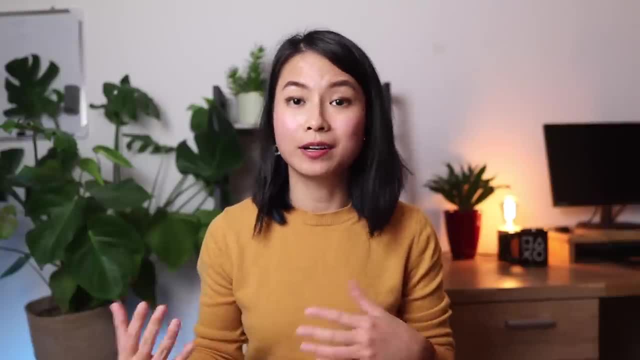 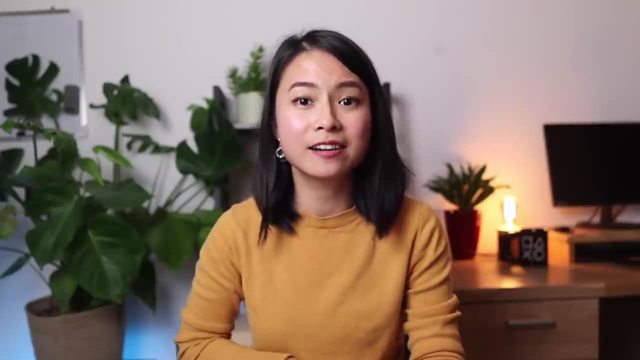 This is also where a lot of companies and organizations struggle. So if you're interested in having an overview of end-to-end machine learning or want to become a machine learning engineer, a great book for this is Designing Machine Learning System. It's a very new book. 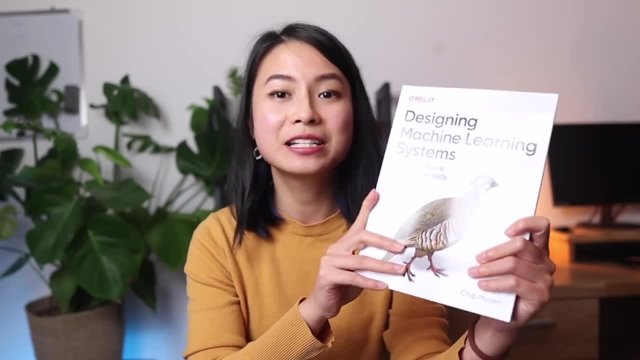 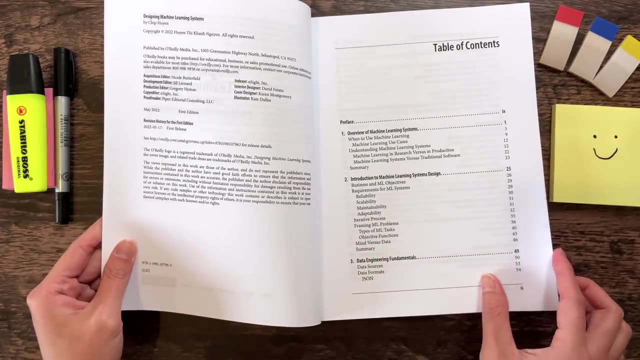 released just a few months ago, at the time of making this video. written by Chieh Huyen, a machine learning researcher who happens to be Vietnamese. This book touches upon many important topics around productionalizing a machine learning system. A model often looks. 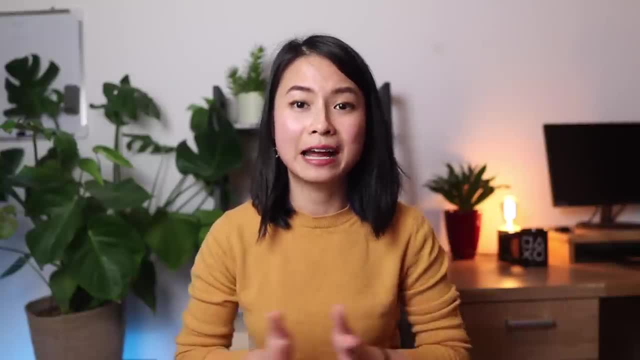 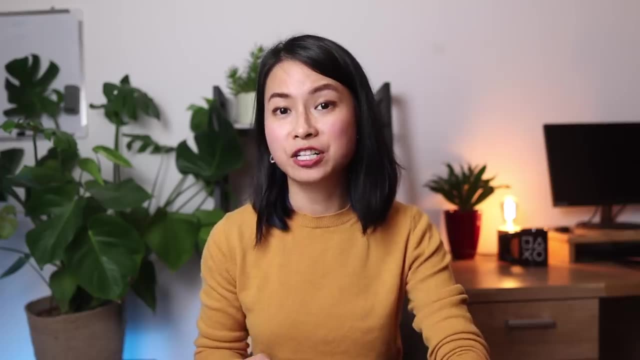 like a data set in Jupyter notebooks, but in various projects at work I have encountered many challenging issues. A very common problem is, for example, class imbalance, When you're predicting financial fraud and only 0.02% of clients in the data actually committed fraud. 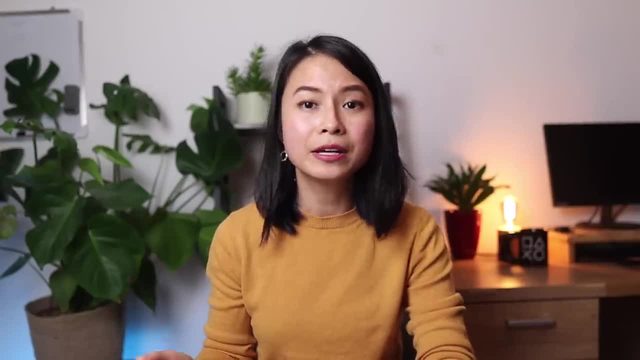 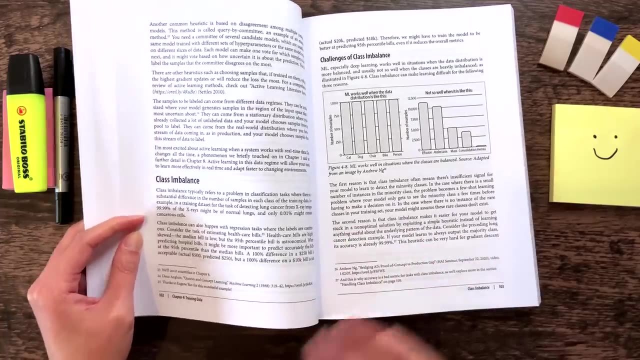 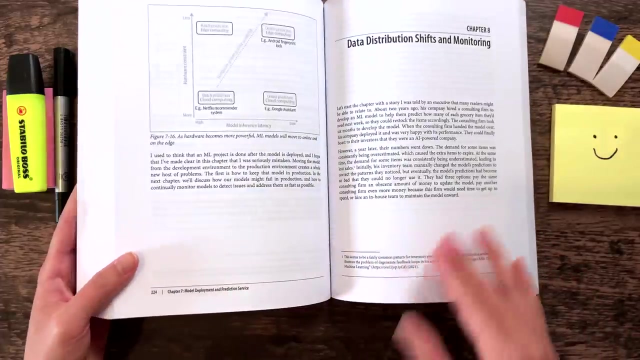 Other times you may not have enough labels to train a model, or you're not sure how often you need to retrain a model in production. All these topics are discussed in this book, in addition to many other topics such as data leakage problem, which is probably one of the worst things in machine learning, and 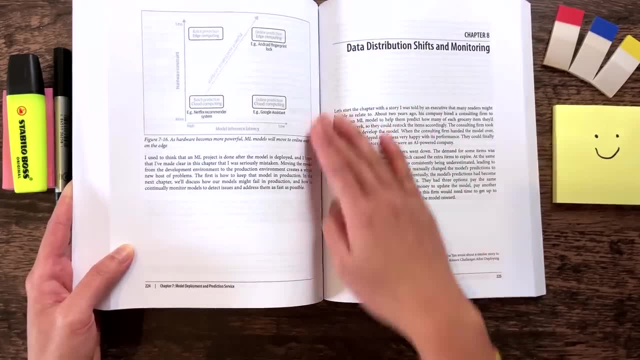 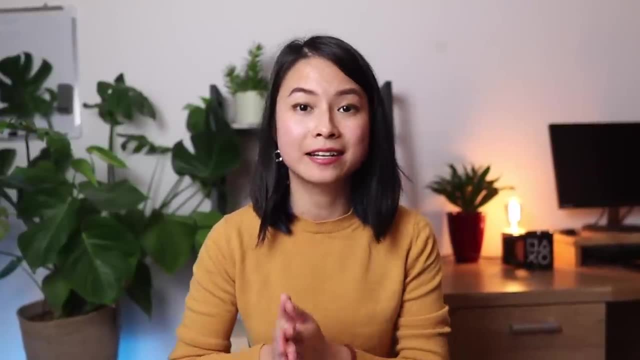 yet surprisingly common. Also, how to engineer good features, how to monitor shifts in the data. The book gives a lot of good examples and derives a lot from the author's experience in industry. I think it so far has been the best in this topic. but some of the claims 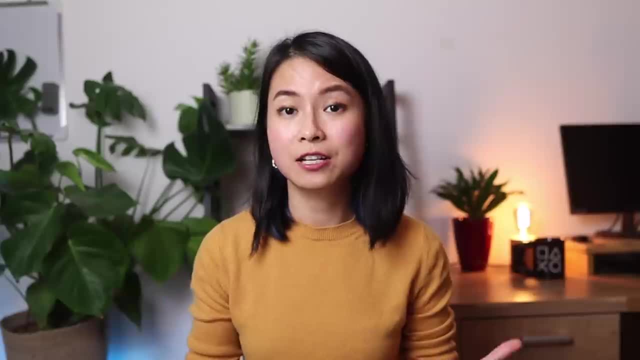 or arguments in the book maybe could be better articulated or backed up with references, just so that for people who don't have a lot of experience or are not experts in the field, it's not a big deal. So if you're interested in learning more about data leakage problems, 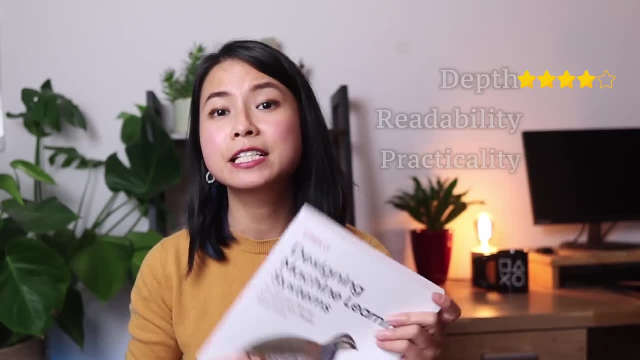 I highly recommend this book If you're interested in learning more about data leakage problems. I highly recommend this book If you're interested in learning more about data leakage problems. you can also follow the discussion, So I'll rate this book 4 stars for depth. 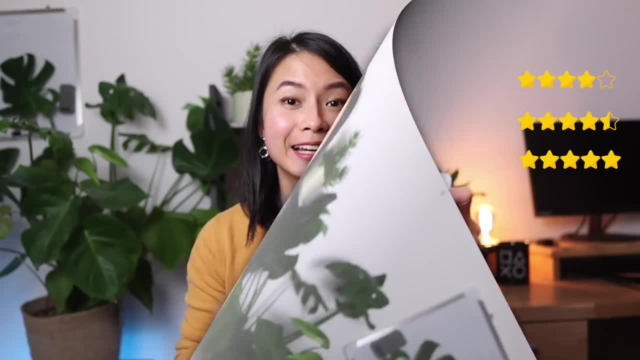 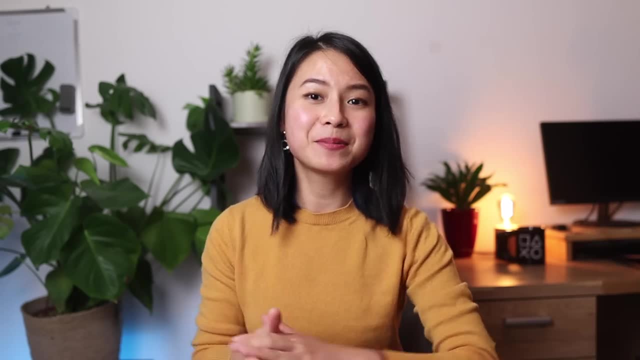 4.5 for readability and 5 for practicality. As we can't talk about data science without talking about data visualization, the next two books will be about data viz. The first book I'll recommend for any data nerds is the book Storytelling with Data. 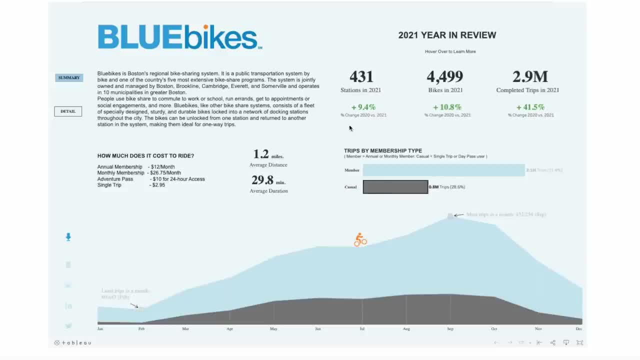 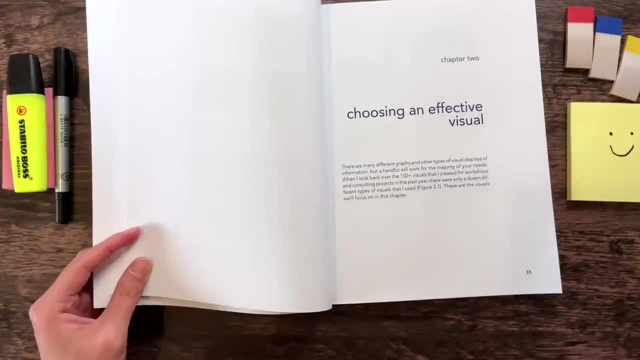 Many of you asked me how to design dashboards and charts. I'll say: read this book first and you'll have a pretty good idea of what's good to do and what's bad to do. There are so many basic principles covered in this book and tons of tips and tricks to think. 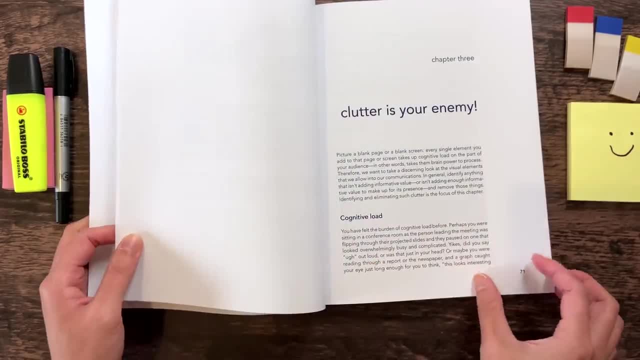 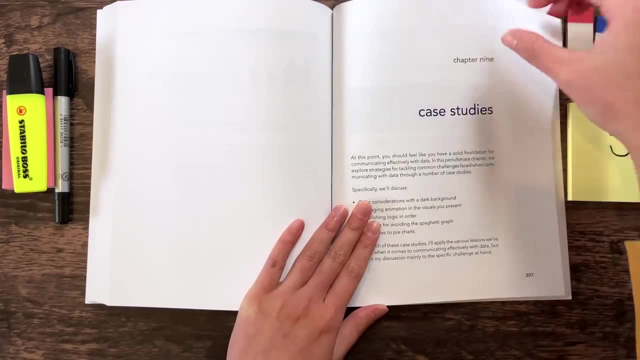 like a designer, putting yourself in the shoes of the audience and catch their attention with your story. I also enjoy the 5 case studies at the end of the book to show you different ways to improve a visualization and tell a better story. So if you ever do data visualization. 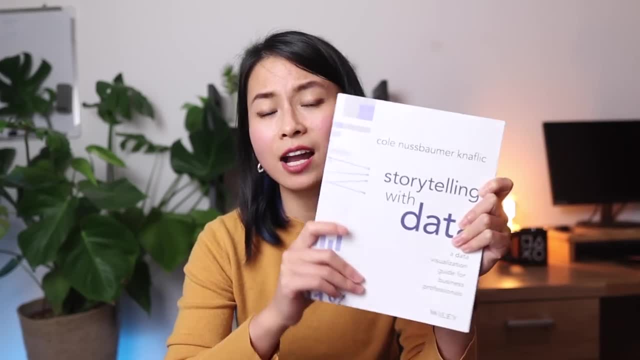 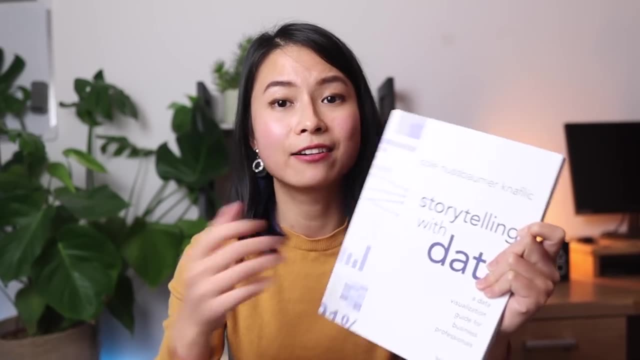 I believe this is the first book you want to read. The only thing I'd love to see more is the advanced or non-traditional types of visualization, and I think this book is going to be very helpful for storytelling. Also, all the examples in this book are static. 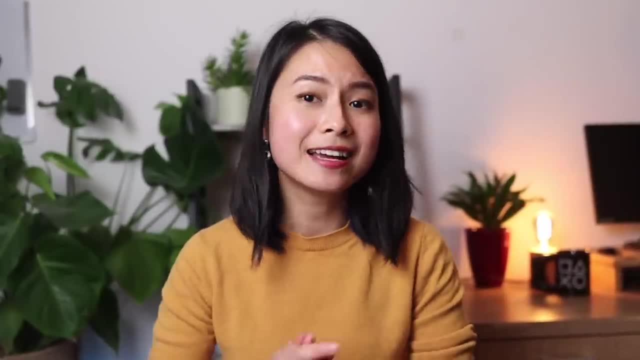 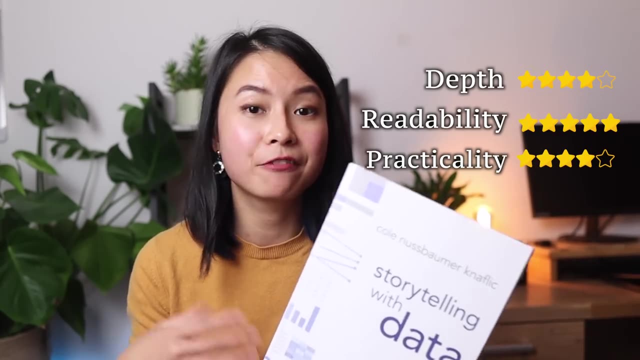 charts. so I feel like the interaction design discussion is a bit lacking in this book. So overall, I'd say this book deserves 4 stars for depth, 5 stars for readability and 4 for practicality. Luke Burrus has a great video where he makes an in-depth review of this. 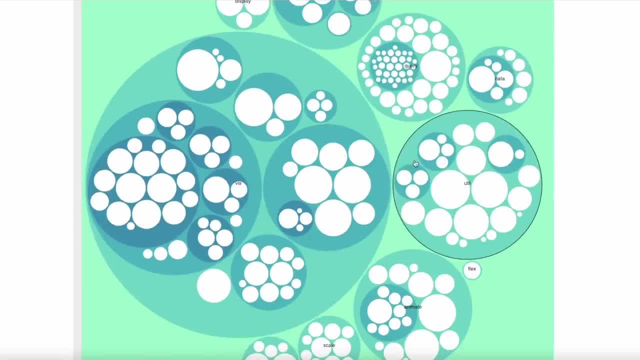 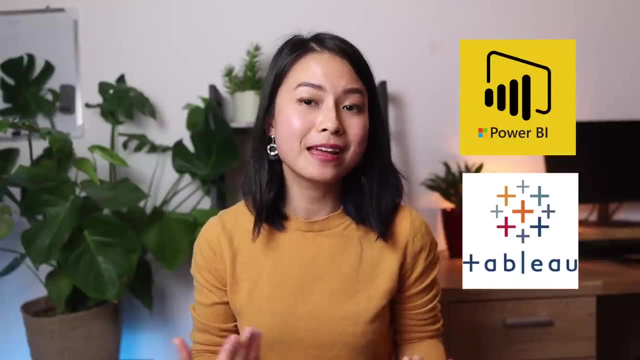 book, so be sure to check it out. Something I'd say I do almost as a hobbyist is data visualization on the web. Power BI and Tableau are great for creating charts quickly, but for me it's still more fun to do web visualizations. 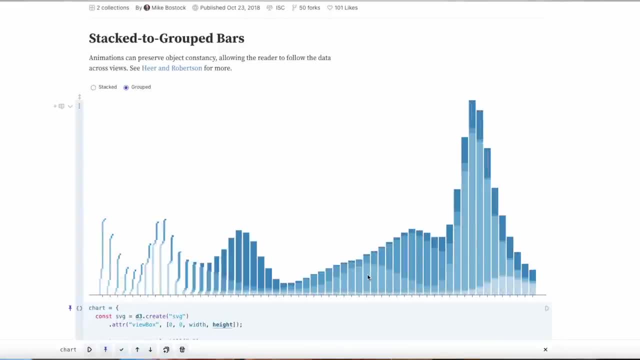 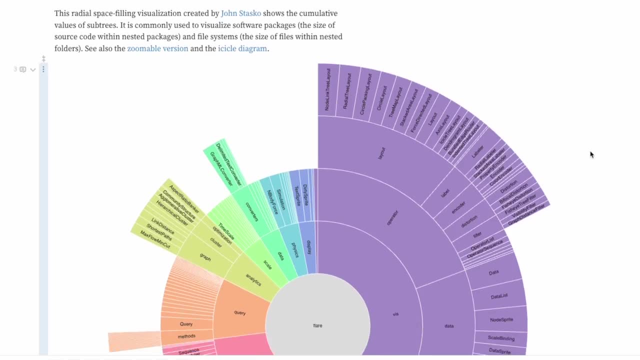 They're more customizable, much more performant because they run on JavaScript. so everything runs very fast and smooth and I can totally break free from the limitations that out-of-the-box software has to offer to create something a bit more pretty and unique. 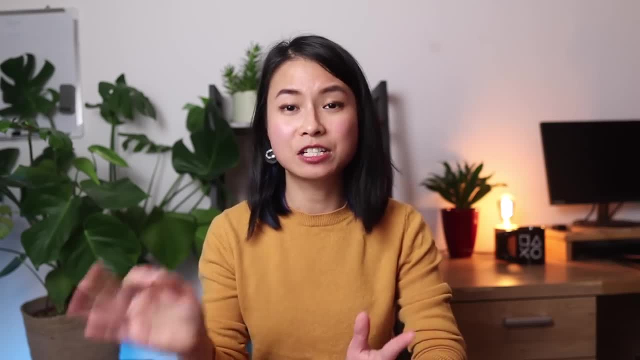 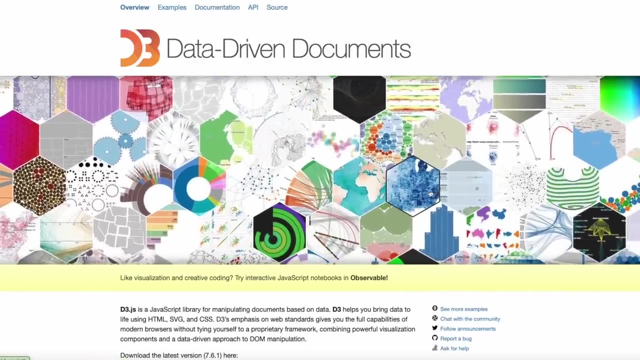 So if you want to go into this rabbit hole of creating browser-based visualizations, I'd recommend the book Interactive Data Visualization for the Web. It's actually about D3.js. You can learn from scratch how to use this library with this book. 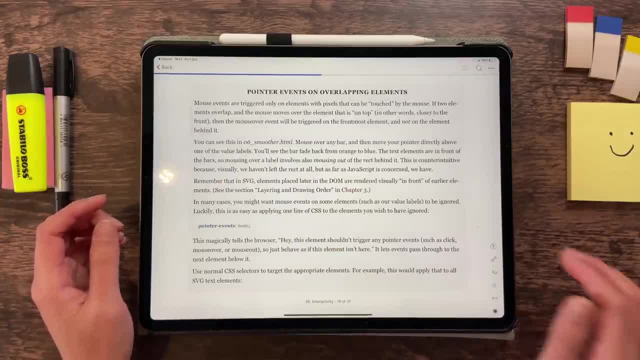 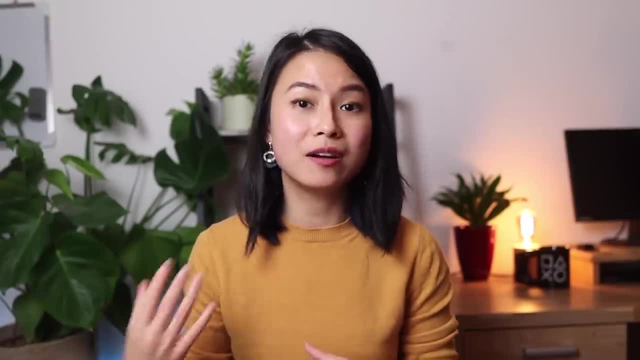 but some basic HTML, CSS and JavaScript would definitely help. That said, D3.js has a bit of a steep learning curve, so I'd say it's more suitable for hobbyists who love creating more complex and pretty graphs. However, we might all agree that 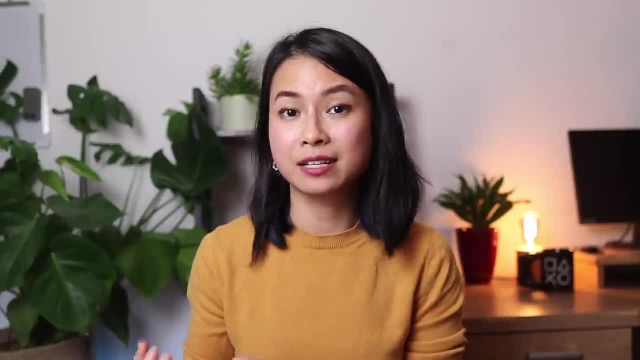 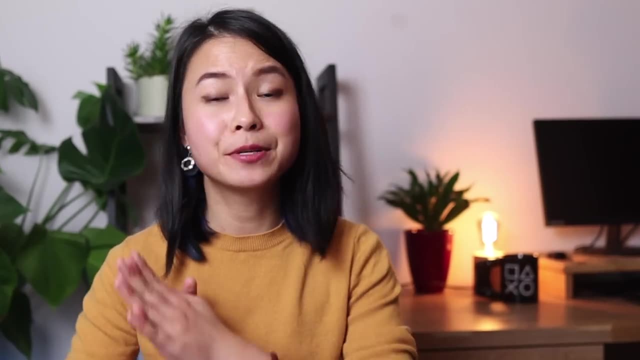 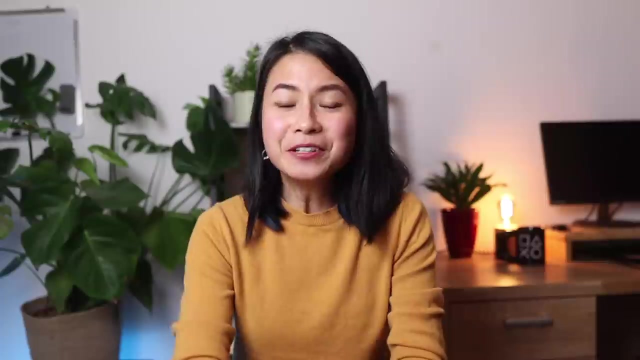 beautiful and performant visualizations often catch people's attention and create the wow effect, and it definitely makes your storytelling more powerful. So overall, this book deserves a 5 stars for depth for the topic, 4.5 for readability and 4 for practicality. 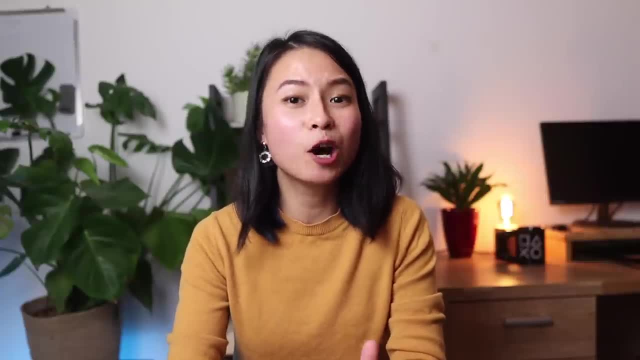 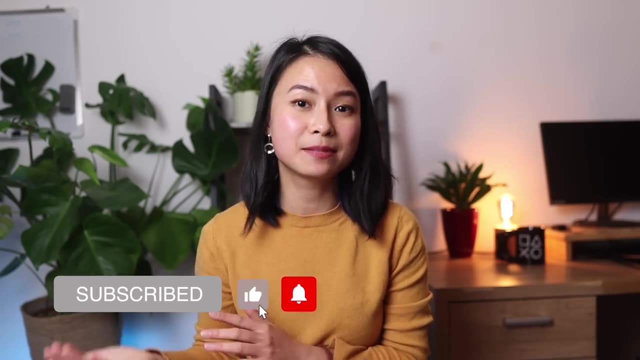 Phew, it was a long video. Thanks for sticking around till now and I hope you enjoyed this video. If you find value in this video, don't forget to smash the like button and share it with anyone who needs book recommendations For video course recommendations for beginners.